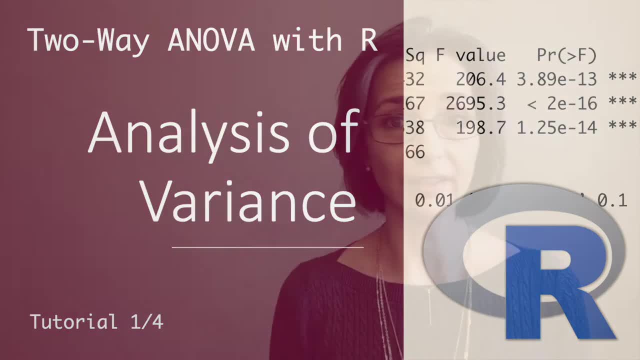 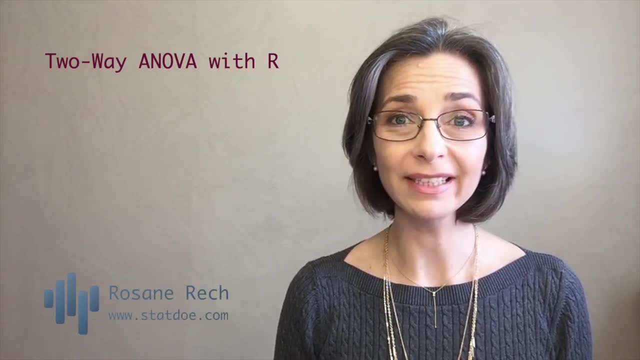 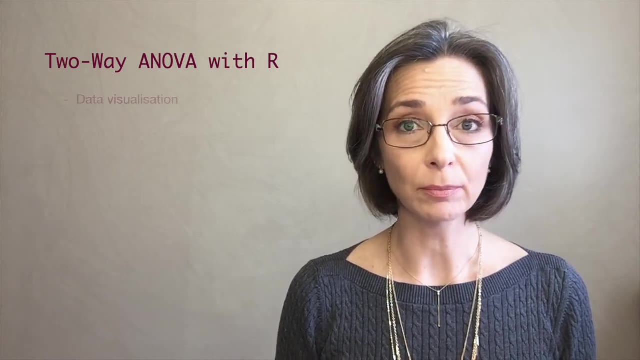 Welcome to the series of tutorials on two-way ANOVA with R. In this series of videos, we are going to perform a complete analysis of a two-factor factorial design. We are going to cover the following steps: Build a simple plot for the data visualization. Perform the. 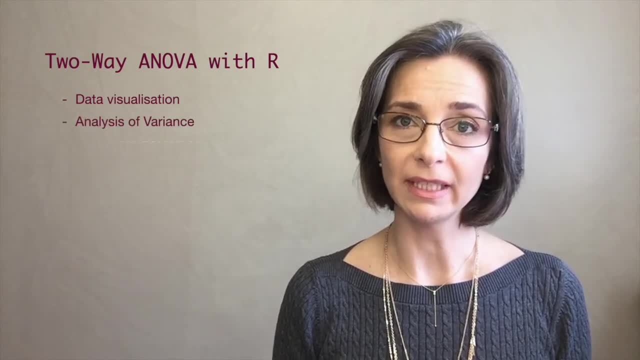 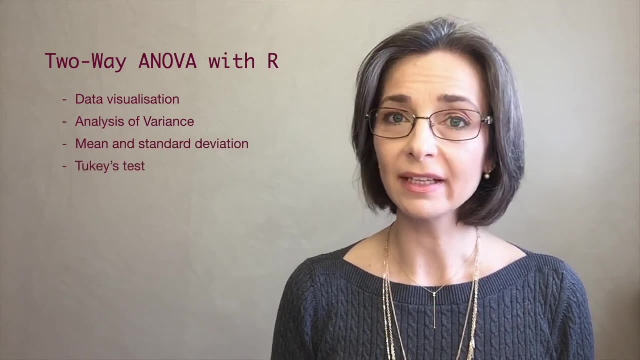 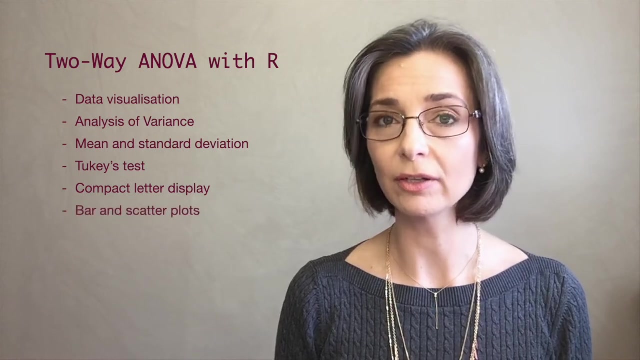 analysis of variants, Create a table with the mean and the standard deviation for each treatment, Compare the means by the case test, Use the compact laser display to indicate significant differences among means And finally, build bar and scatter plots for the final presentation of the results. For more information, we can see the links in the description of. 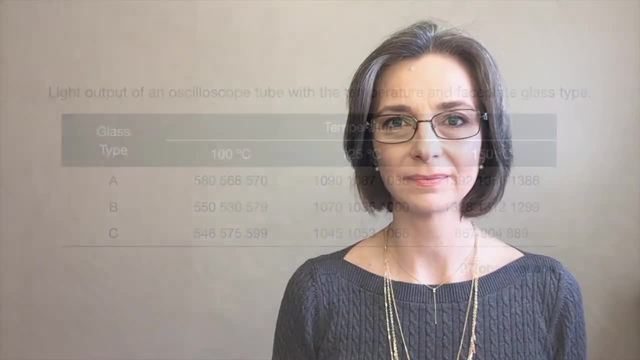 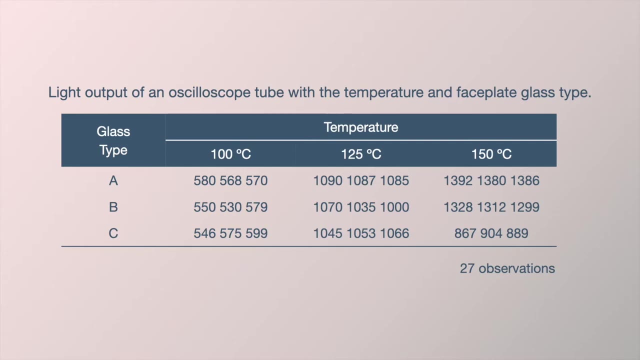 this video. So let's start with the analysis. The problem describes an experiment conducted to study the influence of the operating temperature and the faceplate glass types on the light output of an oscilloscope tube. Three glass types are tested at three different temperatures in a cross-factorial design. The number of 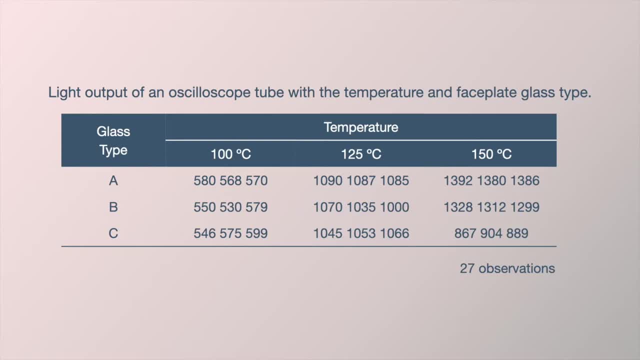 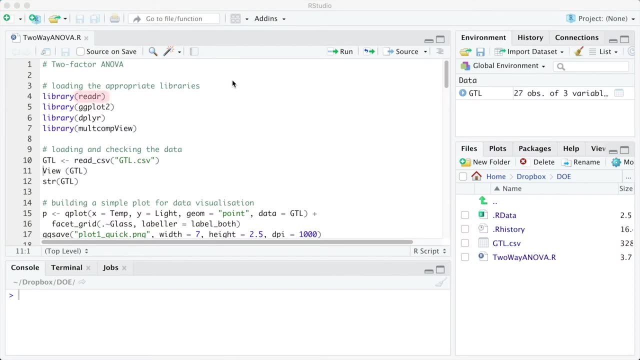 replicates is three totaling 27 observations. We are going to start by loading the appropriate libraries. The reads are to load the data from a CSV file. the digiplot tool for the plots, the deplier for building a table with the 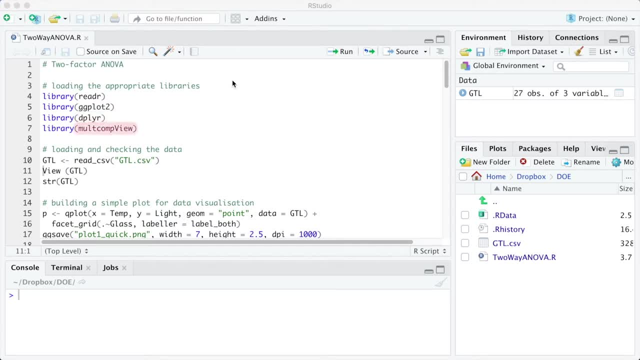 summarized data and the multi-comp view to use the compact ladder display to indicate significant differences in the case test. The first step of the analysis is to load the data file. We will use the view function to open the data as a table and the str function. 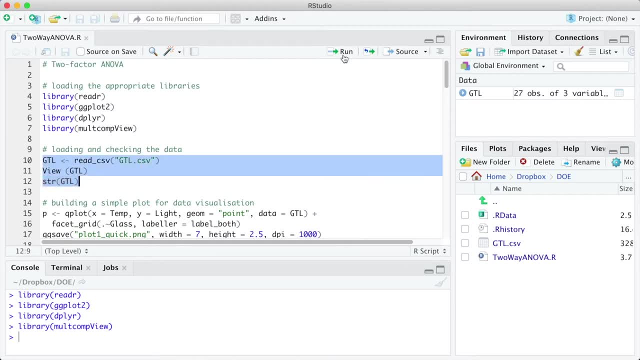 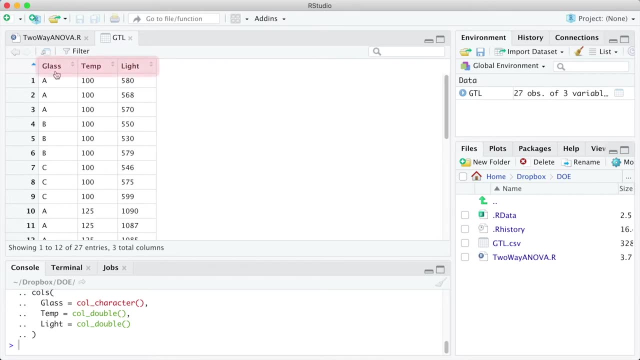 for the file structure. The data file presents three columns: the factors glass and temperature and the response variable light. We can see that we have 27 rows for the 27 observations. Each experimental observation corresponds to a row. In the output of the str function we can see: 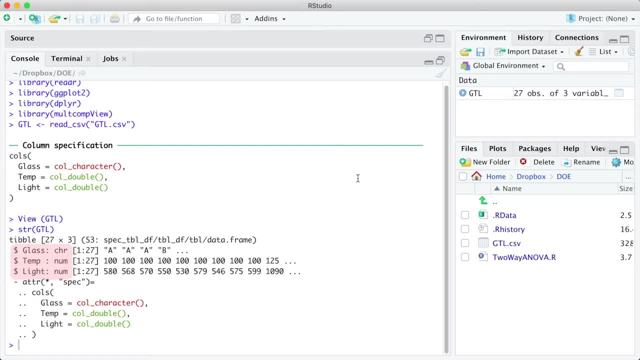 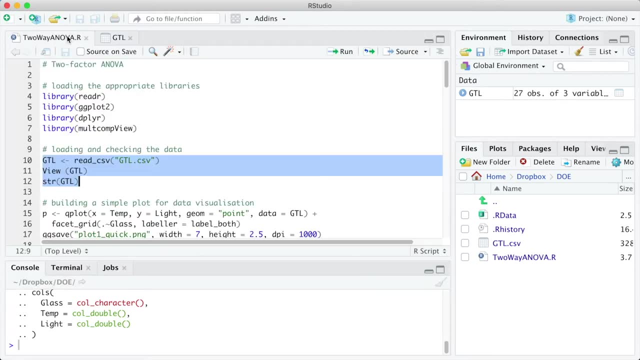 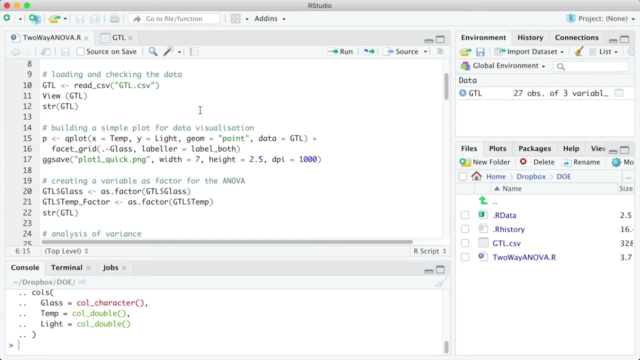 that glass is defined as a character, and temperature and light are non-variable. The data data file takes three columns and factors: glass and temperature. The response variable, light, numeric variables. It is always a good idea to visualize the behavior of the experimental data before diving. 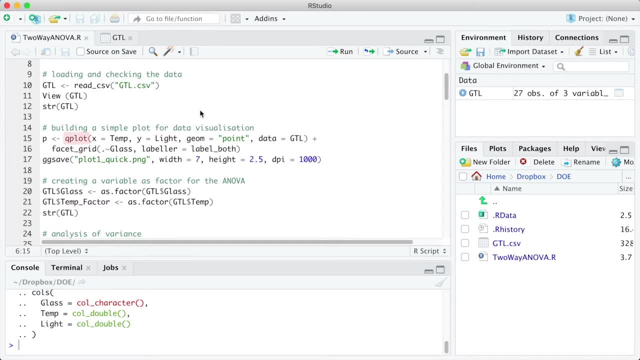 into the analysis. We will use the function quiplot from the digiplot2 library. We are going to build a scatter plot using the temperature as the x-axis, the light response as the y-axis and splitting the plot by the faceplate glass type. 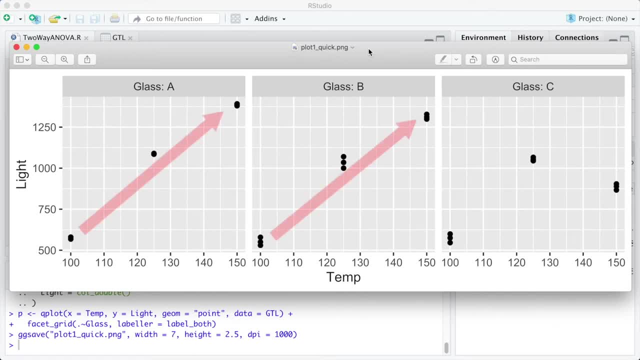 We can see that the light output increases with the temperature for glass types A and B. However, glass type C has a maximum at 125 degrees. The plots indicate that we will probably have at least the temperature and the interaction between temperature and glass as significant. 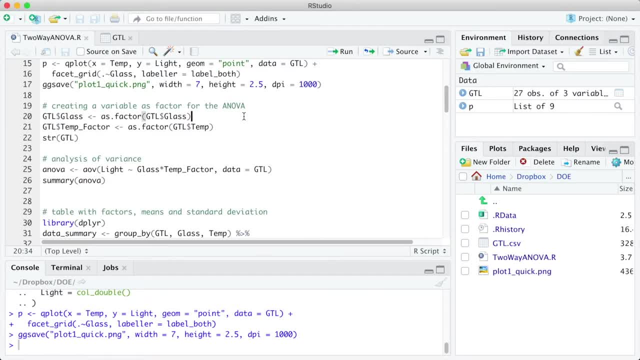 For the analysis of variance or building an OVA table. we need to have the independent variables in the data file defined as factors. For glass, which is defined initially as a character, we will convert it into a factor For temperature, which is a numeric variable, we will duplicate it, creating 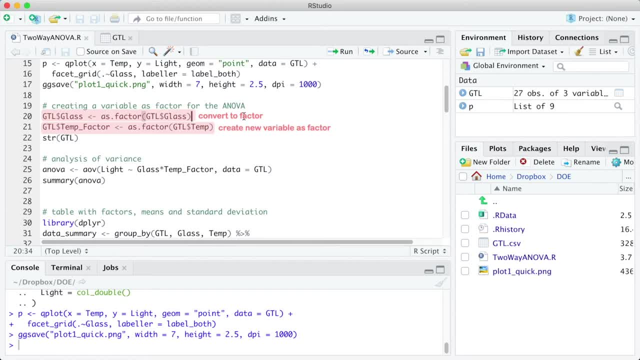 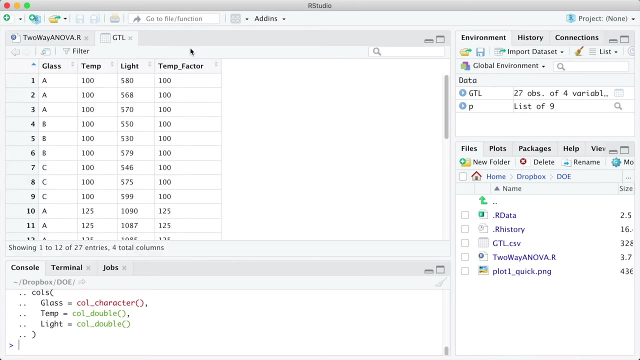 a new variable, tempFactor, defined as factor. We are not going to convert it because we may need it numeric for further analysis or plots. We can see that the data file has a new column, tempFactor, defined as factor, and we kept. 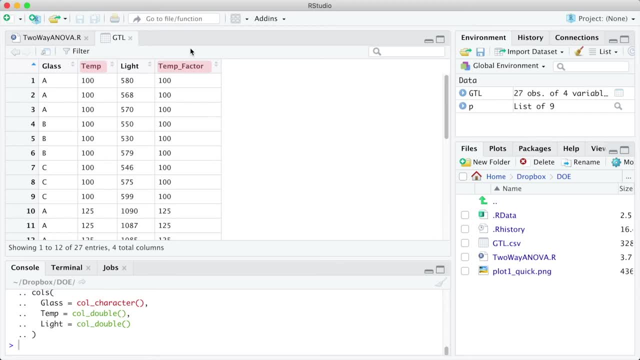 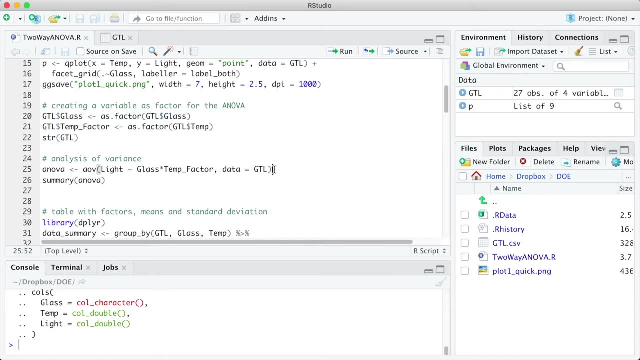 the original variable temp as numeric. The next step is to perform the analysis of variance During the AOV function. the Coat shows we are going to run the ANOVA for the Light over response variable as a function of factors: Glass and temperature.